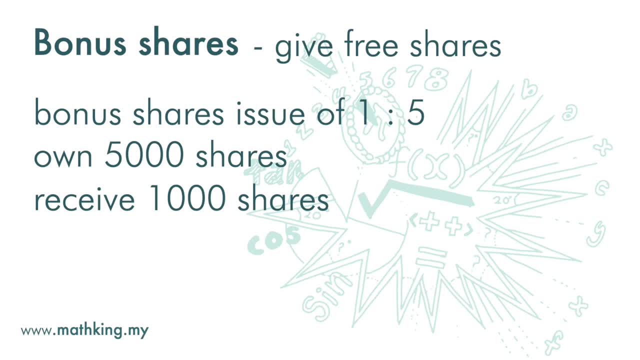 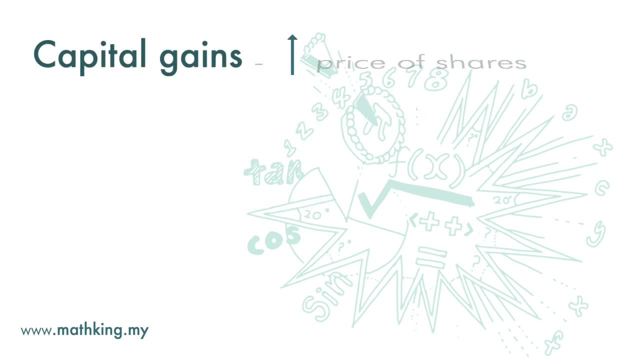 Lastly, even if a company does not issue dividends or bonus shares when it makes profit, you will still gain from the increase in the price of the shares of the company, because the share price of a company that makes profits is likely to increase and you can sell your. 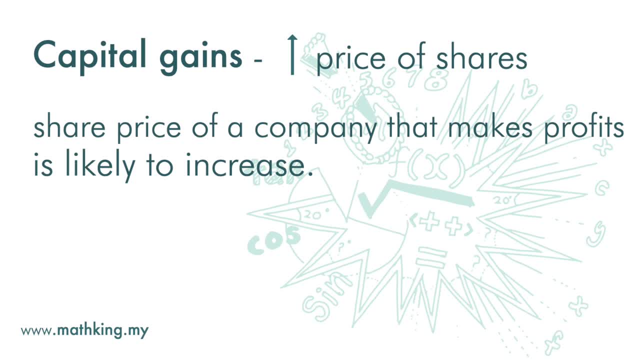 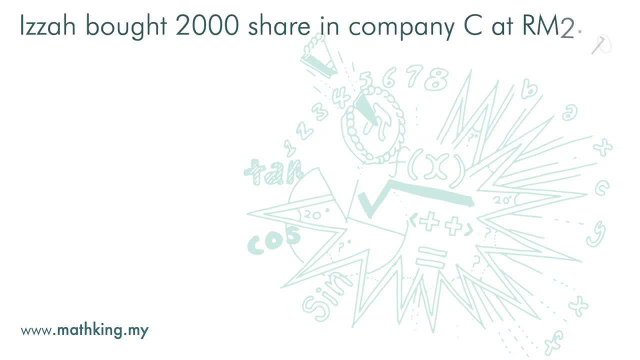 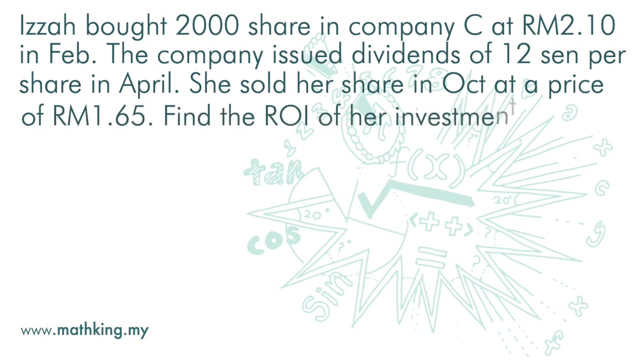 shares to realize your gains. Now let's look at this question. Iza bought 2,000 shares in Company C at RM2.10 in February. The company issued dividends of 12 cents per share in April. She sold her shares in October at a price of RM1.65. 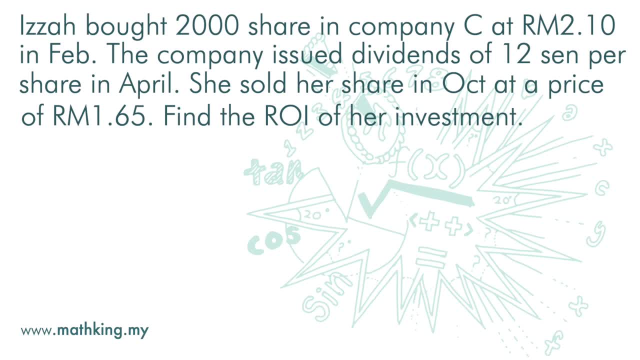 Find the ROI of her investment. Cost of investment is RM2.10 times 2,000 shares, Which is RM4,200.. The dividends she received was 12 cents times 2,000 shares, Which is RM240.. The capital loss is RM2.10 minus RM1.65 times 2,000 shares. The total loss is RM2.10 minus RM1.65 times 2,000 shares. The total loss is RM2.10 minus RM1.65 times 2,000 shares. The capital amount of 5,000 shares in an apartment is 4,年 5,000 Korean Won, which. 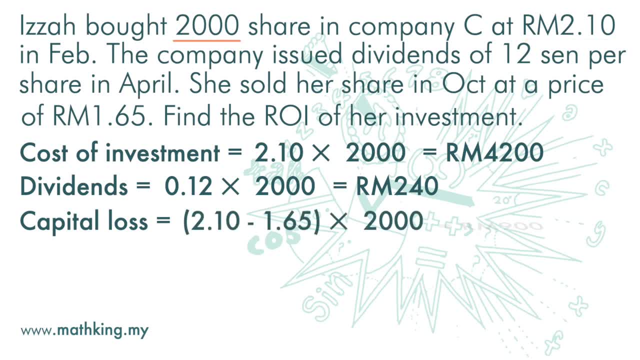 is RM2.10 minus 2,000 shares, which is RM1.65 times 2,000 shares. The total difference is RM2.10 minus 2,000 shares. Rk1 cost of across the investment of 5,000 shares. 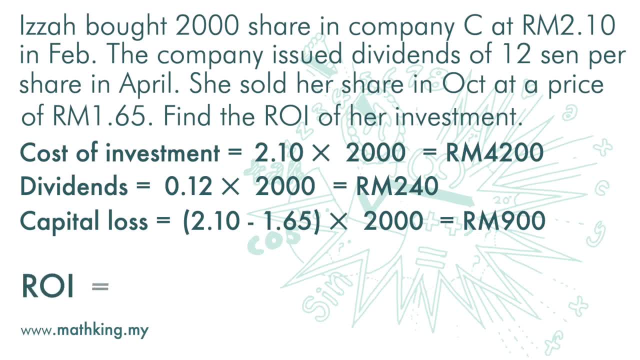 The final investment fills Rk1. as this sum plus the capital loss size, The final investment fills Rk2, as which is so we have 2A-9하, The final investment fills Rk1 as such rk2 chance. 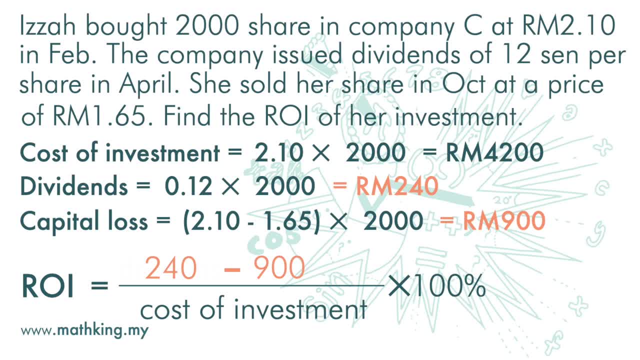 As the capital of the shelf is drugs. So the capital of the shelf is drugs. If I remember correctly, Iza bought 10 shares in saying: and the total described value of the 6 dolla is 2A-zy grandpa아ă ◔. such that se at 0,对.